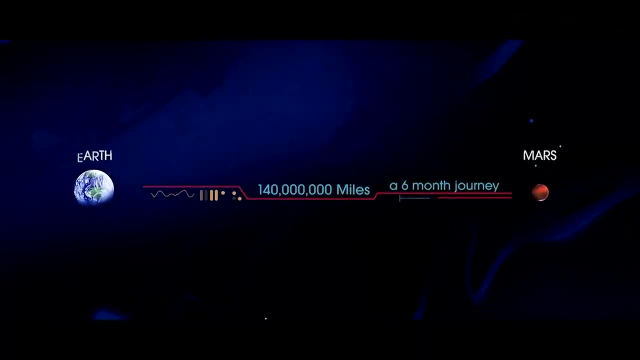 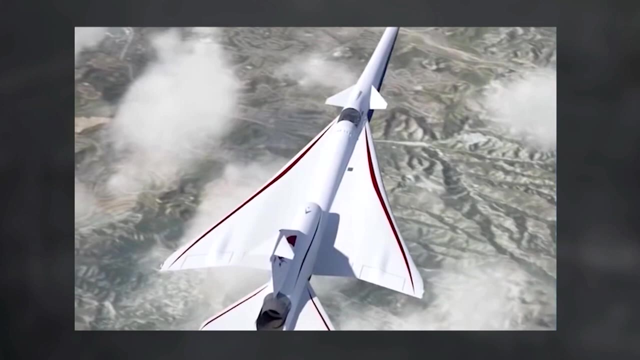 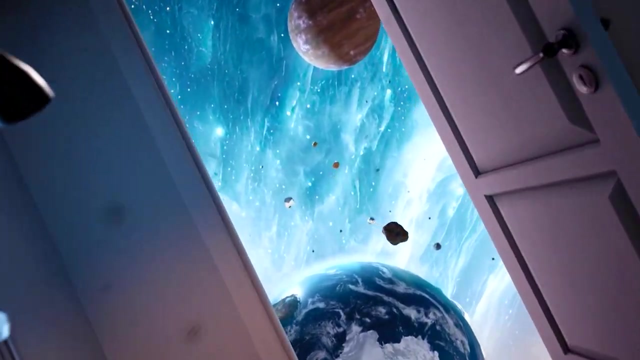 of returning humans to the moon and eventually onto Mars. advanced materials will be equally important in protecting the lives of our astronauts, earth-based flight vehicles and human life here on Earth. Unlike most who are inspired by what we do at NASA, it wasn't dreams of. 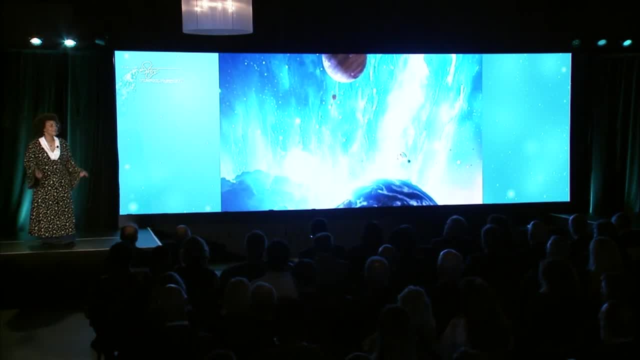 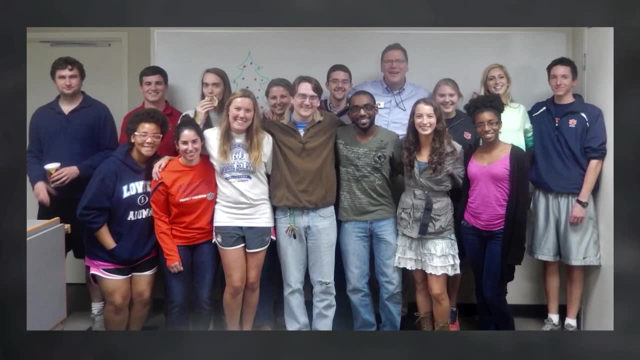 space or being an astronaut that steered me here. It was NASA's first A Aeronautics that got me excited about pursuing this career. I started college as a studio astronaut. I had the pleasure of studying aviation at art major with no desire to go into any engineering field, but I knew I loved. 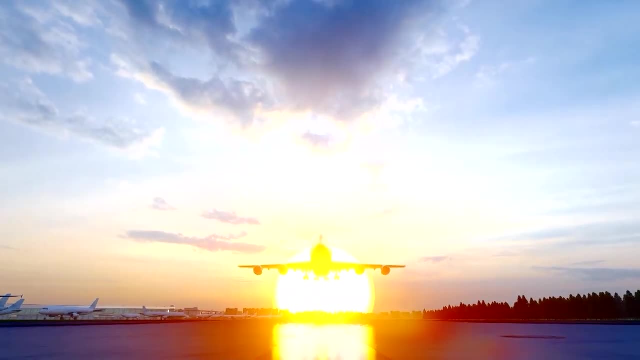 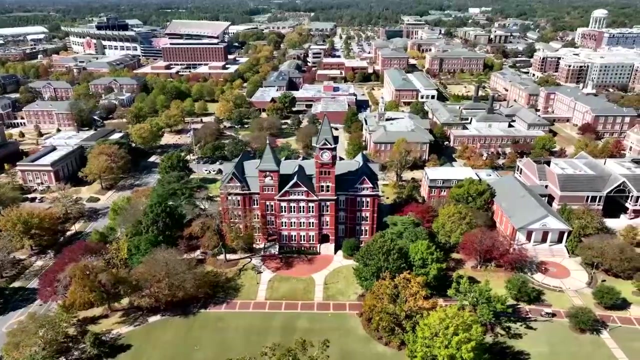 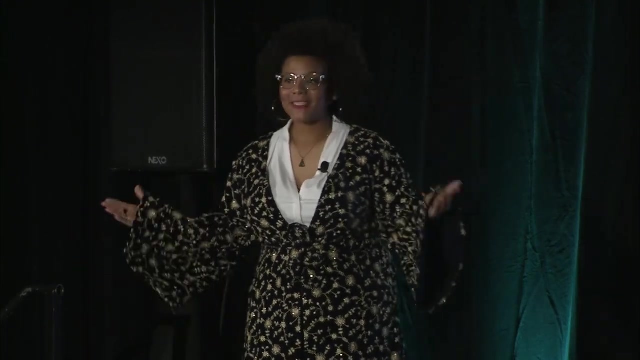 flying. I loved traveling and I loved how flight made my world bigger and the rest of the world smaller. so when I changed my major to physics at Auburn University, I was left bewildered, not knowing exactly what future career I'd want. then I came to NASA Glenn as an undergraduate intern and I was able to work on. 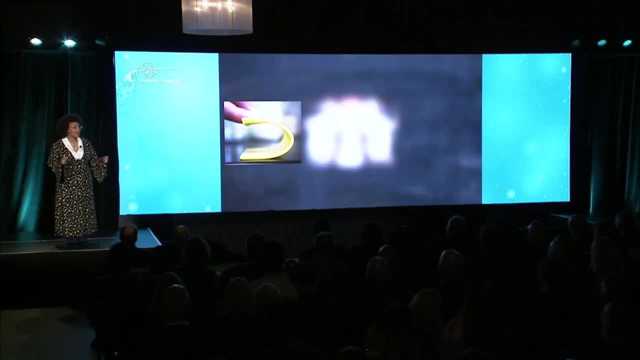 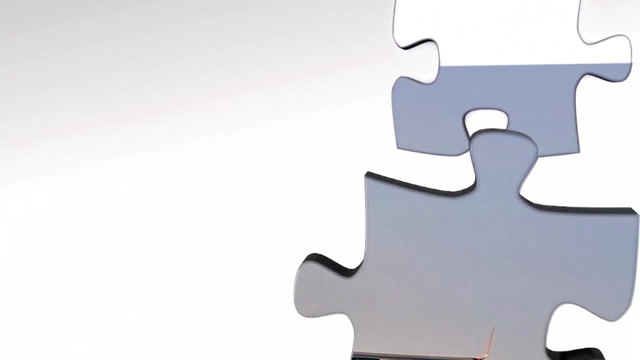 aerogels, which are very unique, lightweight, highly insulative materials for thermal protection systems for vehicles like the Space Shuttle and other high-speed flight vehicles on earth and in space, and at that time it was like I had found the missing piece of the puzzle of figuring out what I 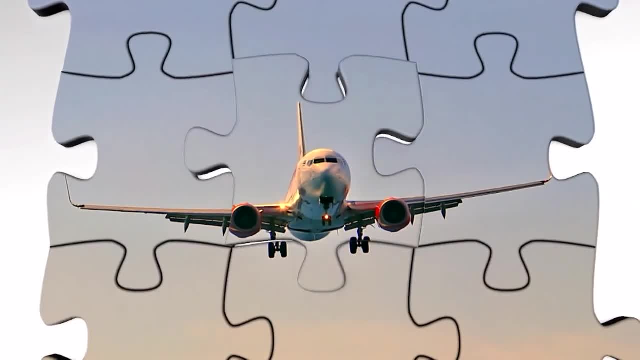 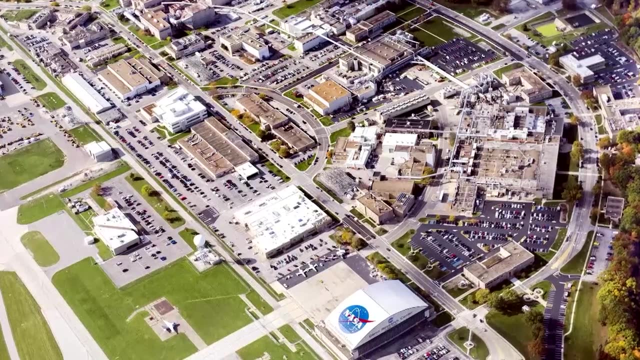 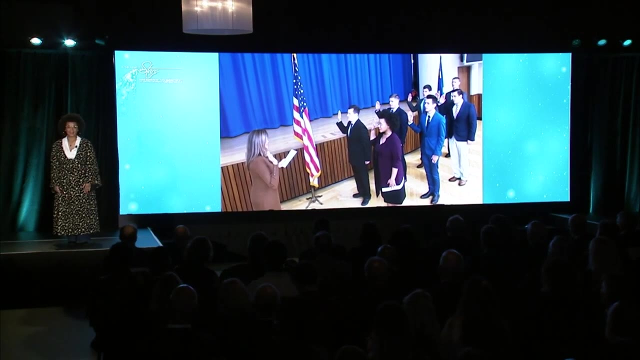 wanted to achieve with my life. I wanted to work on advanced materials to protect human flight systems, and Cleveland was where I needed to be to accomplish that goal. once I started graduate school in Pennsylvania, I was awarded a graduate fellowship through NASA Glenn and I became an employee as a pathways. 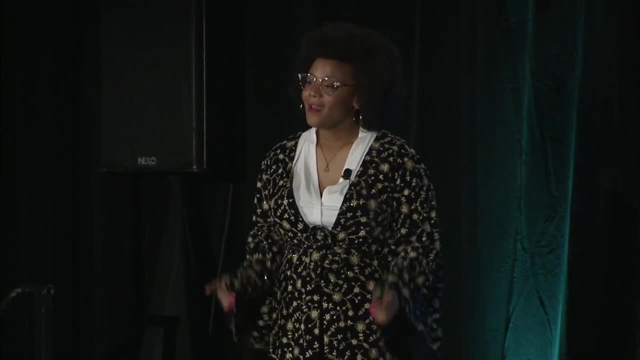 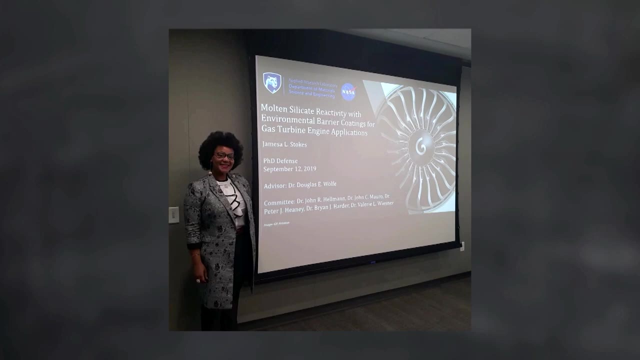 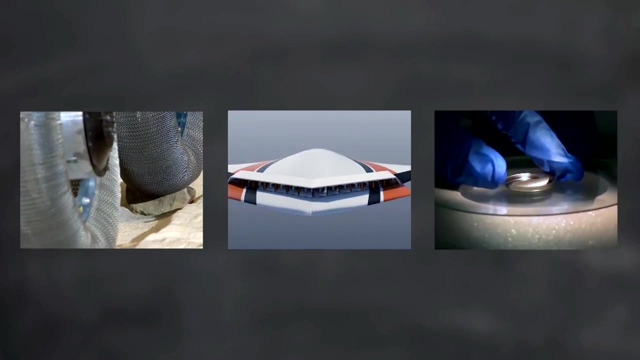 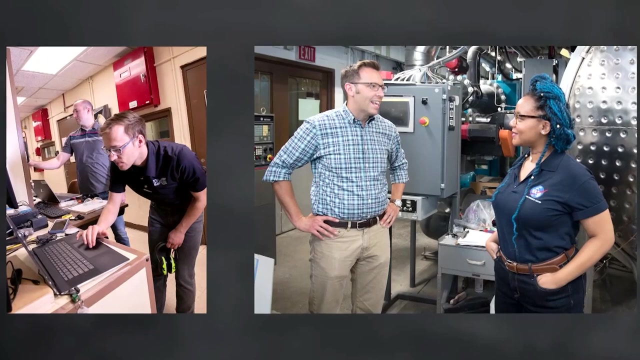 intern right before I defended my thesis that aerogel research that set this once inexperienced intern on the path to NASA was just one example of the vast amount of influential work accomplished at Glenn Research Center. and today my team and I are continuing that tradition of innovative materials research in a number of ways. some of our current 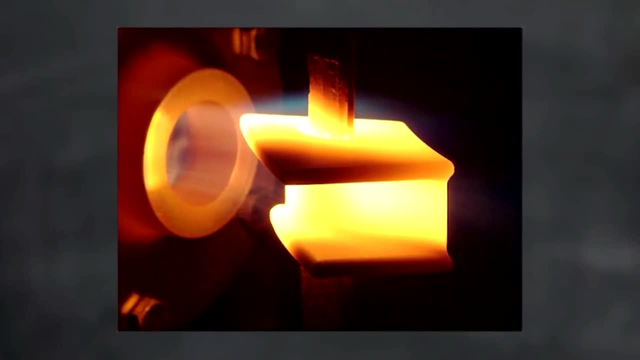 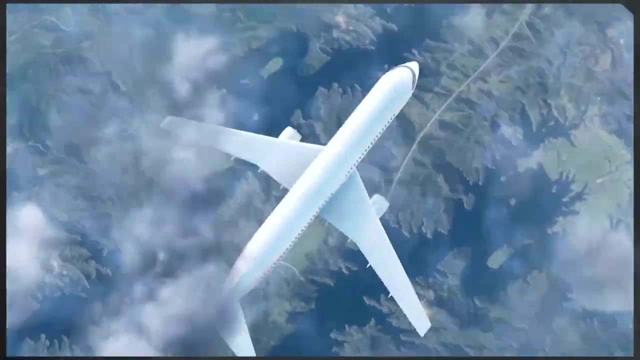 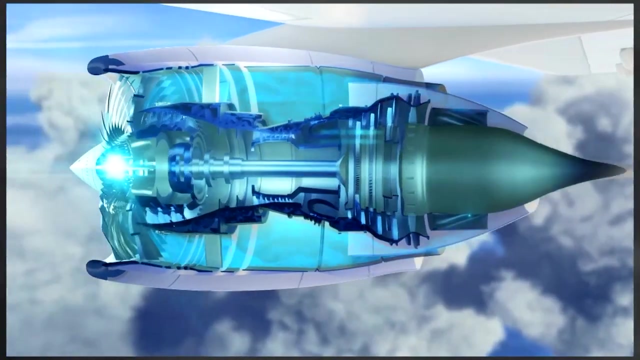 research involves environmental barrier coatings, which are used to protect gas turbine engine components from their corrosive environment. it's important to protect these components, as our nation's next-generation airplane engines will run at higher temperatures to improve fuel efficiency and reduce harmful emission products. decades ago, the first generation of these coatings were 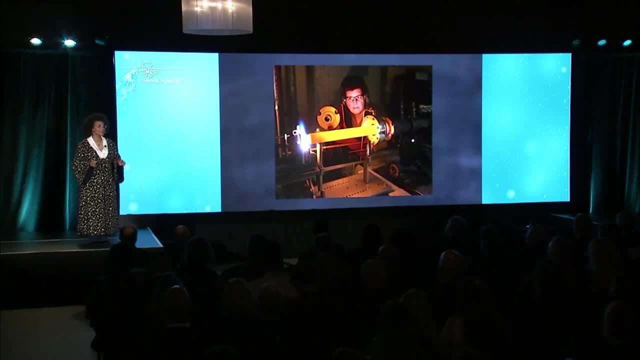 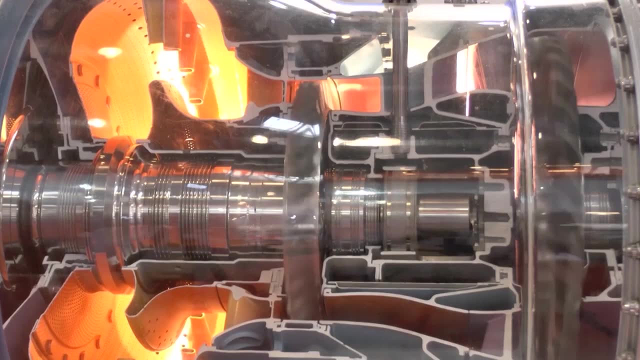 developed right here at NASA Glenn, and we're here today to talk about the things that we know we need to do to protect our planet. we're here at NASA Glenn in Cleveland and now my team and I are pushing state-of-the-art technology in current engines. today I'm excited to help develop coatings and lighter weight. 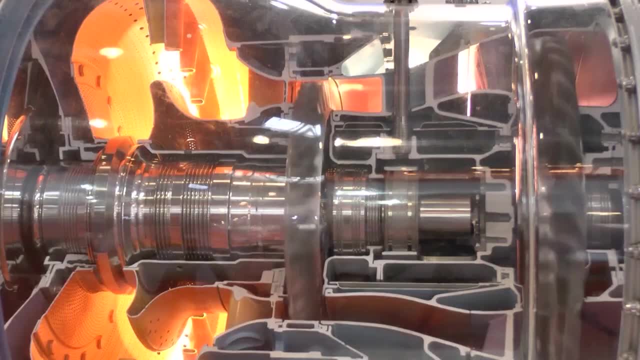 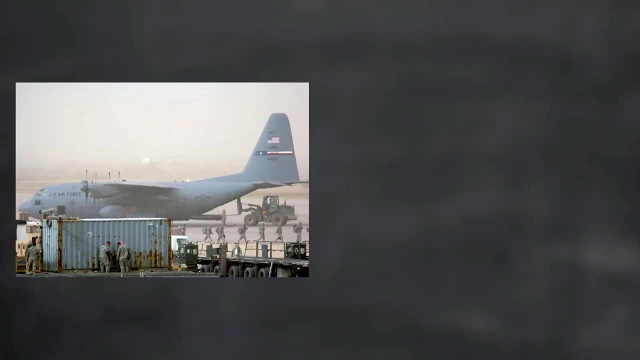 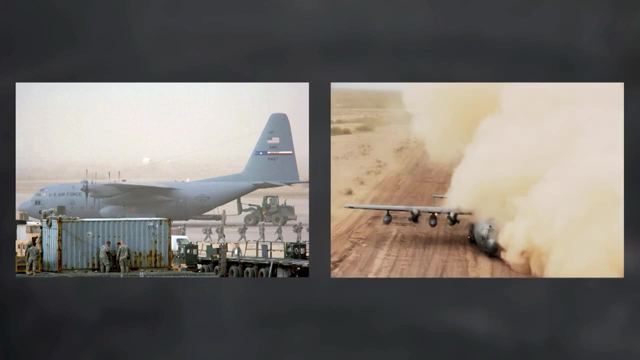 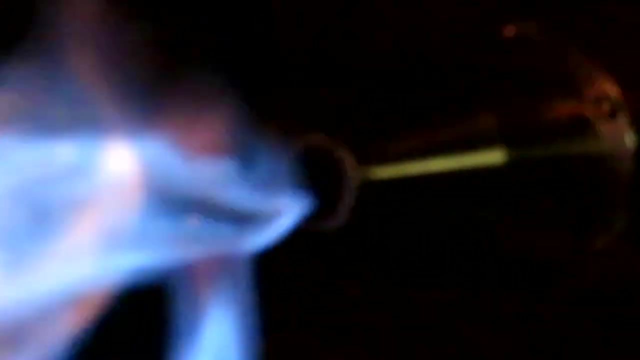 materials to help replace heavier metallic engine components. during engine operation. we investigate how these coatings and components fail, whether it's by corrosion caused by combustion products like water vapor, or by particle deposits caused by ingestion of desert sand or volcanic air, or by the use of. We collaborate with commercial engine companies to qualify their materials for flight readiness in our testing rigs that can reach temperatures above 3,000 degrees Fahrenheit. 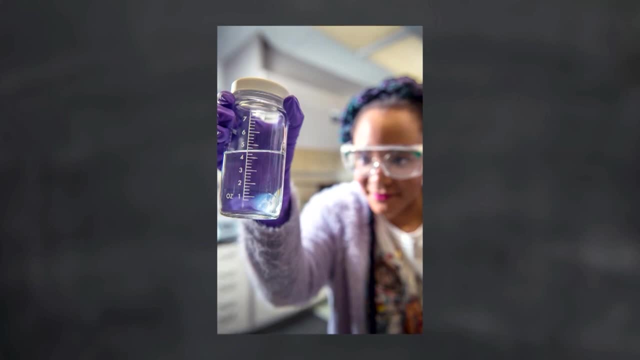 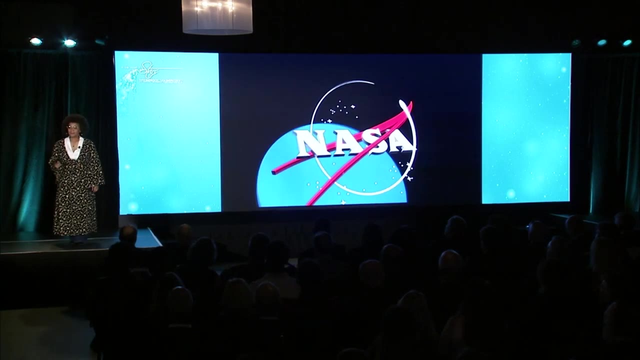 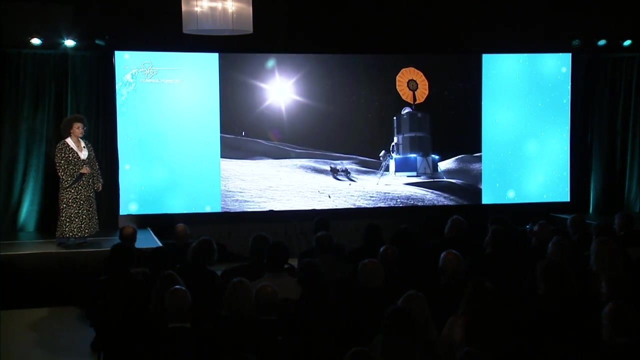 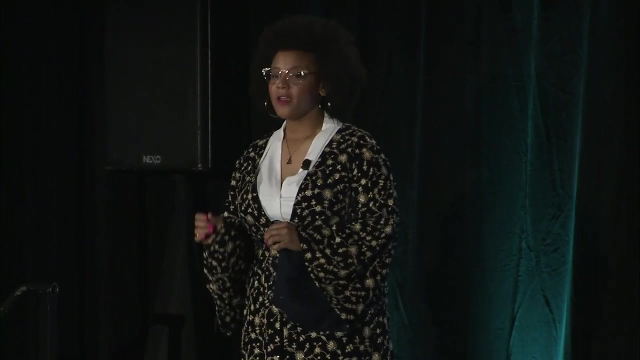 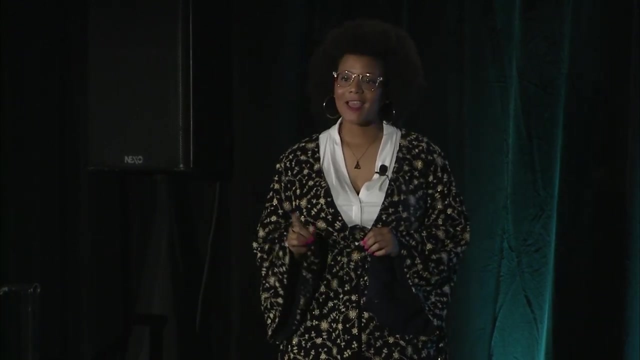 But we also never forget the fundamentals of basic materials characterization and new materials discovery. On the space side, the S in NASA, we are investigating lunar dust mitigation strategies for structures on the moon and eventually on to Mars. The Apollo missions taught us that one of the greatest challenges is how to remove very fine, highly charged dust particles from surface materials like solar panels, space suits and helmet visors. 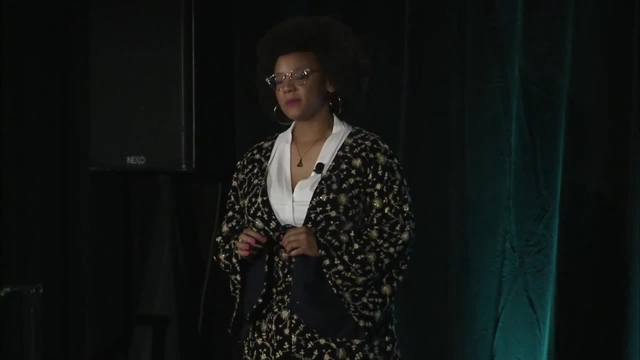 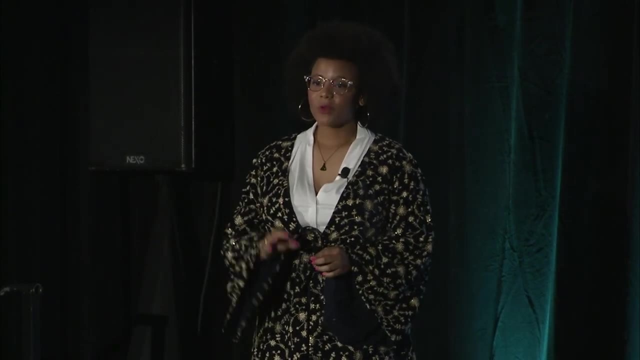 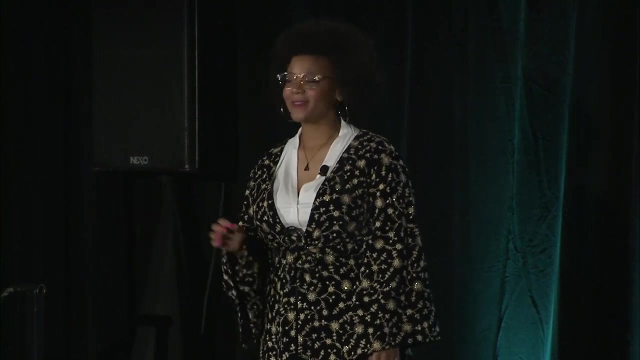 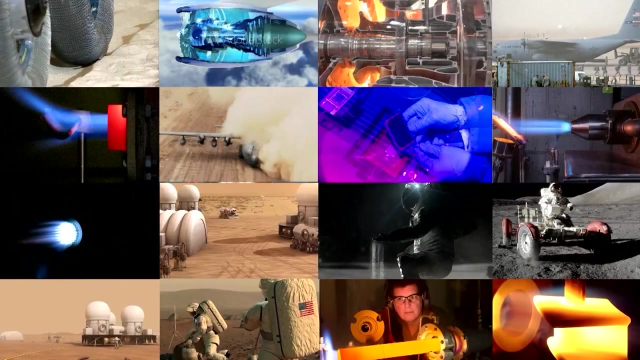 Dust compromises the functional integrity of these materials, And so we are investigating. We must develop better removal technologies, such as anti-adhesion coatings, brushes or electric discharge techniques, if we are to effectively live and work on other planetary bodies in our future. I've highlighted just a few of the many technical achievements and challenges we face in our pursuit of pushing the limits of what we can accomplish. 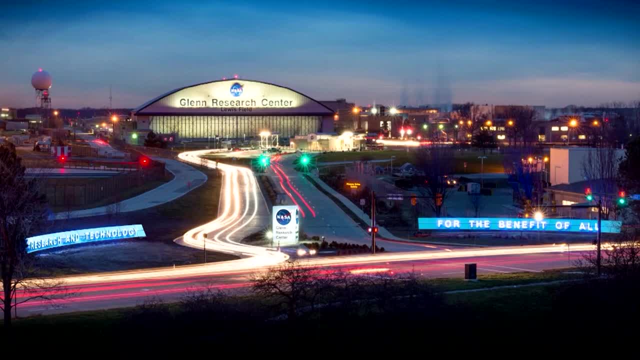 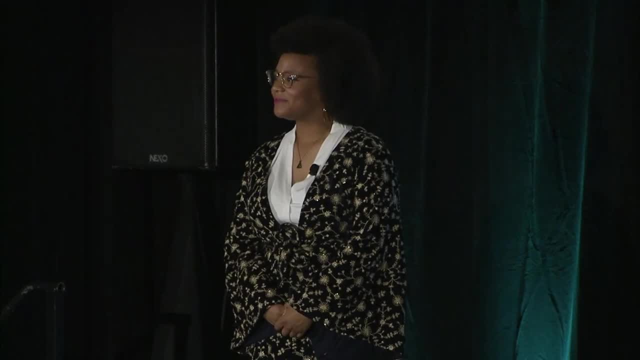 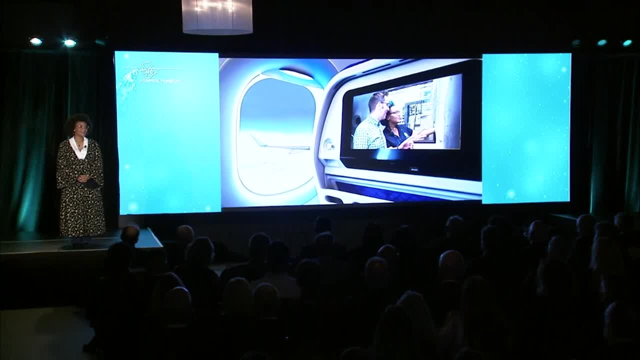